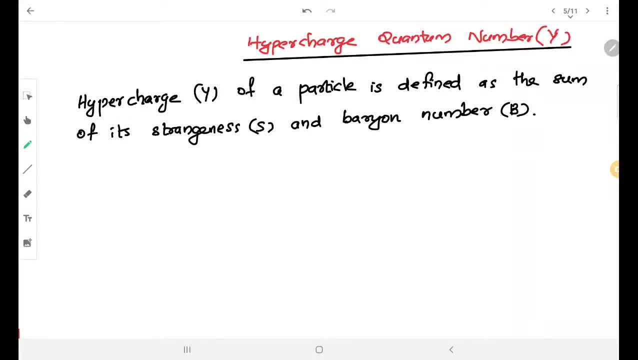 Dear students, today we are going to discuss about hypercharge, quantum number. What do we mean by hypercharge? Hypercharge is denoted as y. Hypercharge of a particle is defined as the sum of its strangeness and baryon number. 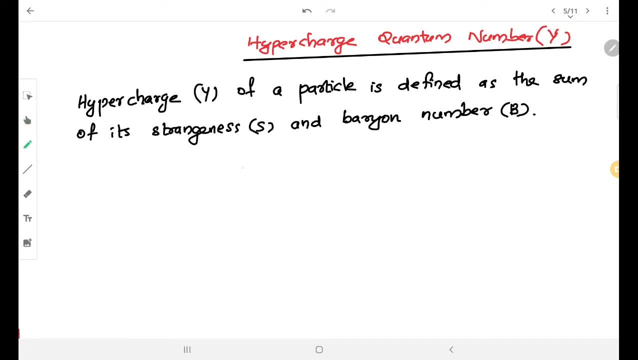 So it is easy to denote. It is denoted as y. y is equal to b plus s, where b is the baryon number and s is the strangeness. We know that. which are the strange particles? We already discussed in the last class about strange particles. 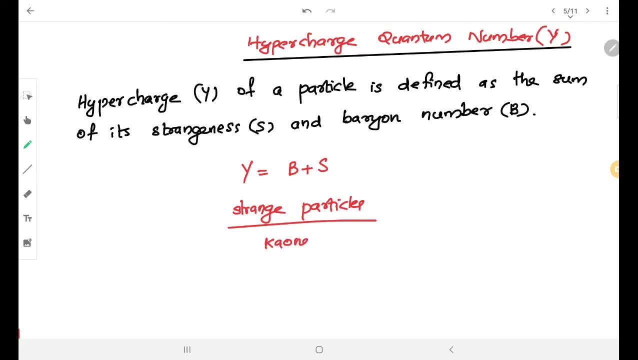 Strange particles family include kions, Kions have strangeness value plus 1 and hyperons have s values Lambda 0, sigma family, psi family and omega minus Sigma 0 has s minus 1.. Sigma family has s minus 1.. 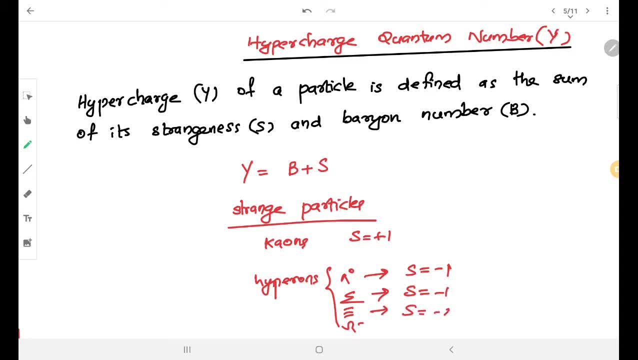 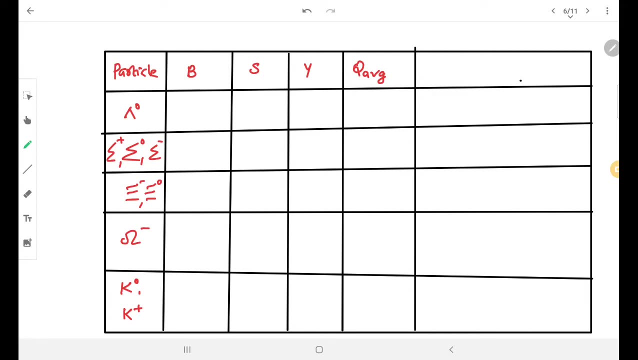 Psi family has s minus 2 and omega family has s minus 3.. So all these families have strangeness, So they have corresponding hypercharge also. So we can see the examples. So let's see the hyperon first. Lambda 0 has. lambda 0 is a hyperon, It is a baryon. 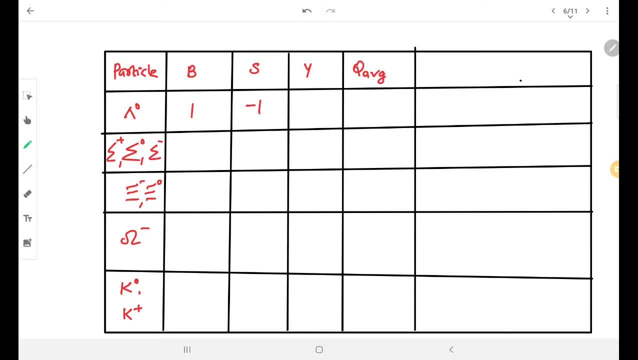 So its baryon number is 1.. Its strangeness is minus 1.. So its value of y, So its hypercharge, is 0.. Okay, Now what is the average charge? How we can find the average charge. Average charge means if a family consists of one member, its average charge is same as the charge of that member. 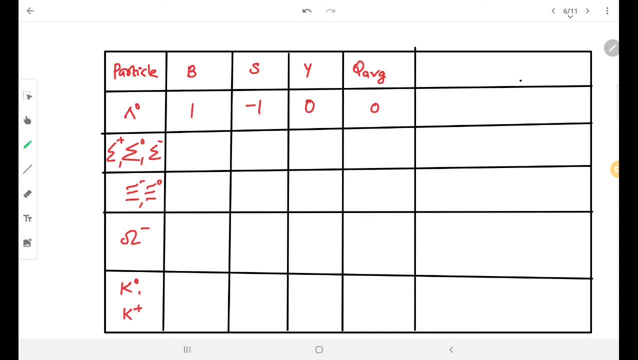 That means here the average charge is 0.. Now in the case of second family, that means sigma family. Sigma family consists of three members. First member, Sigma family, has charge 1,. second charge has number 0, and third charge has number minus 1.. 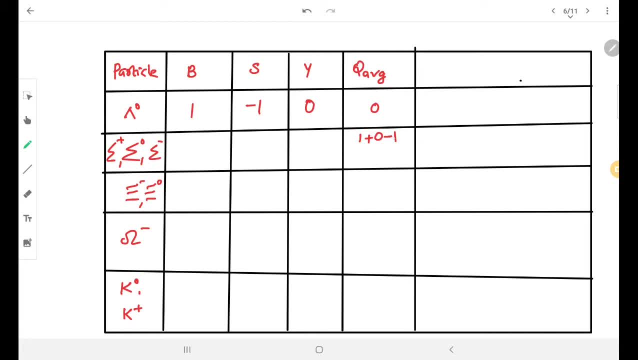 So the average of these three charges is 1 plus 0 minus 1 divided by 3.. Because there are three members in the family, So average charge is like this: In that family all the members' charges are added Sum of all charges corresponding to all members in that family divided by total number of particles in that family. 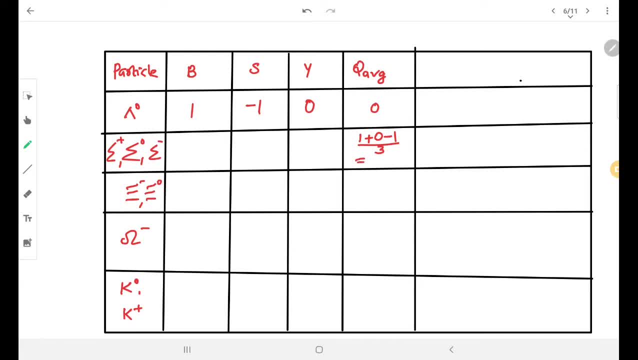 Or total number of members in that family. So what will come here? This is also. This is also 0.. Okay Now, sigma family's barrier number 1, strangeness minus 1.. So their hypercharge is also 0. 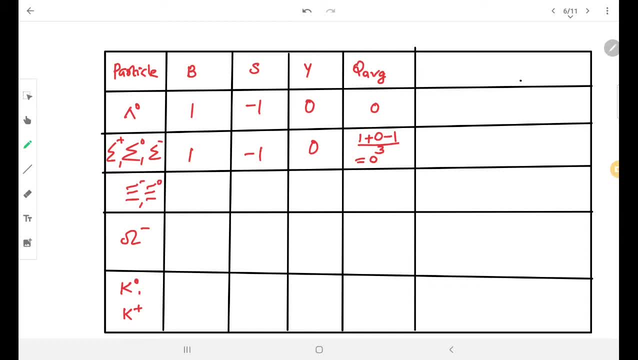 Now psi minus, Psi minus and psi 0. They have barrier number 1. Strangeness minus 2.. So y is equal to b plus s, y equal to b plus s. So 1 minus 2, that is minus 1.. 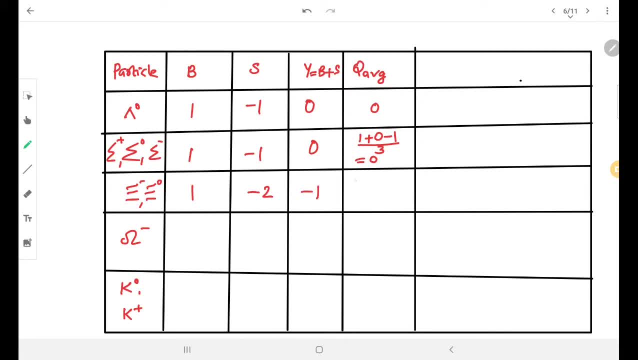 What is the q average here Here? psi minus has minus 1 charge And psi minus has minus 1 charge. So psi 0 has 0 charge divided by 2.. So what is the average charge of psi family? That is equal to minus 1 by 2.. 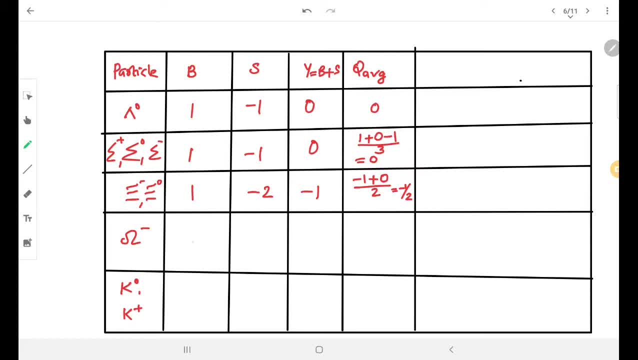 Now omega minus. Omega minus of barrier number 1. Strangeness: minus 3.. So y is 1 minus 3.. That is minus 2. This is the hypercharge of omega minus. And what is the average charge? Average charge is: 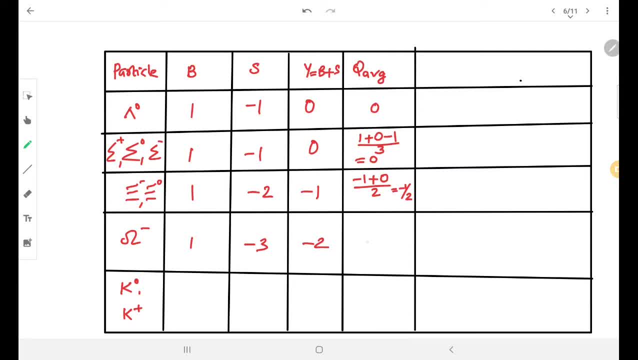 Average charge is minus 1.. Because only one member and it has charge minus 1.. Because only one member and it has charge minus 1.. Because only one member and it has charge minus 1.. Next is kion family? Kion family barrier number is 0.. 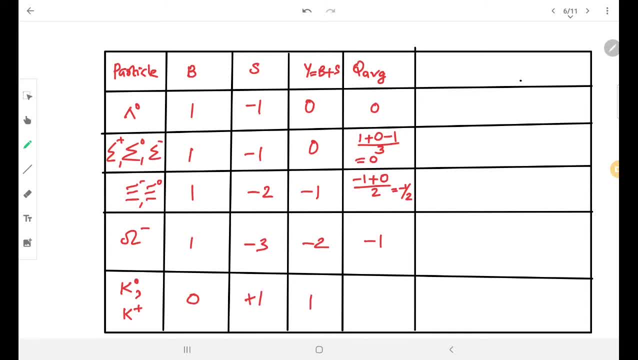 Strangeness is plus 1.. So what is y? y is 1.. What is the average charge? Average charge is 0 plus 1 divided by 2.. That is 1 by 2.. So these are the. This is the case of hypercharge. 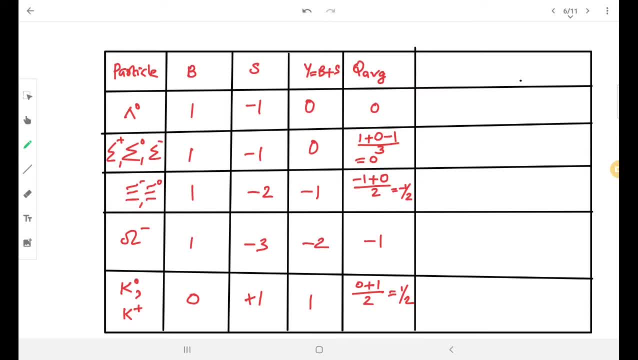 In the case of hyperons and kions, For all other baryons Which are not strange particles, They have y value 1.. For example, In the case of proton, In the case of proton, Baryon number, strangeness and y. 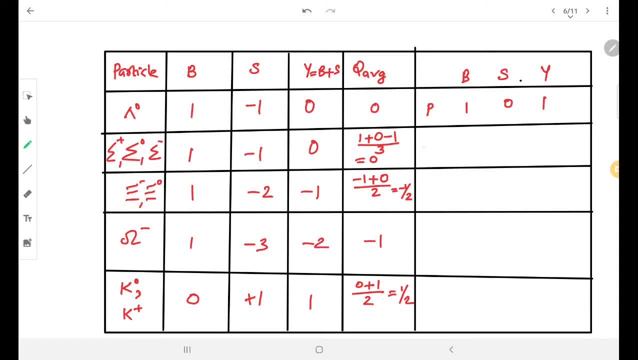 Baryon number is 1.. Strangeness is 0.. So hypercharge is 1.. In the case of neutron, So in the case of nucleons, Proton and neutron, The y hypercharge is 1.. Baryon number is 1 and strangeness is 0. 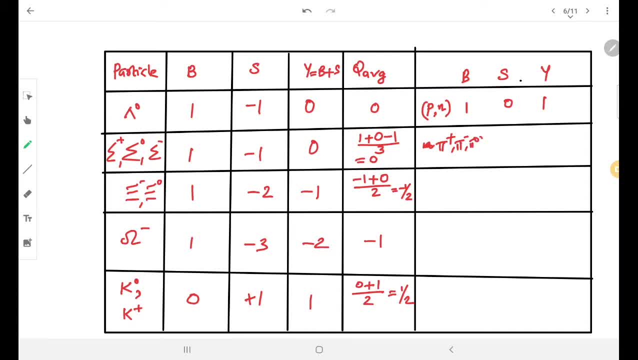 Similarly, in the case of pi plus, Pi minus and pi 0. That is pion family. Strangeness is 0. So hypercharge is 0.. Similarly we can find The hypercharge of all particles If we know the baryon number and strangeness. 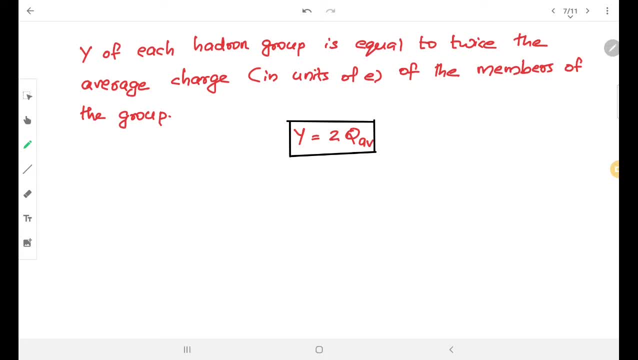 Ok. So next important point of Point regarding this hypercharge is that Hypercharge of each hadron group Is equal to Twice the average charge. Average charge is always expressed in units of e. E is the basic unit of charge. 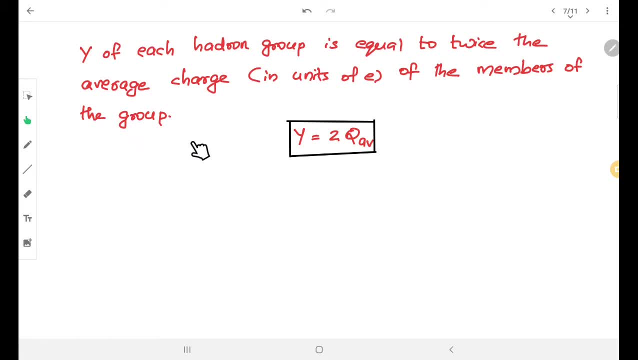 So average charge of the members of the group. That is One hadron group. Hadron means baryons and mesons, So the hypercharge of one hadron group Is equal to Twice the average charge of that group. Ok, 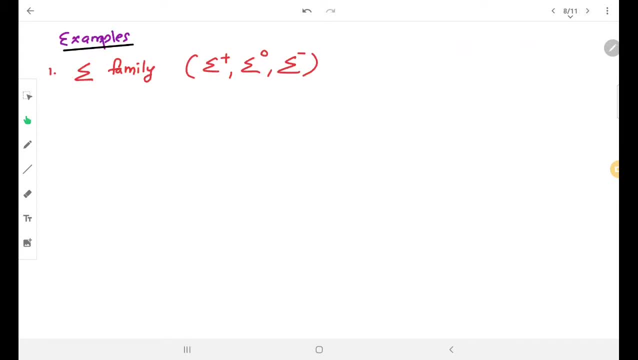 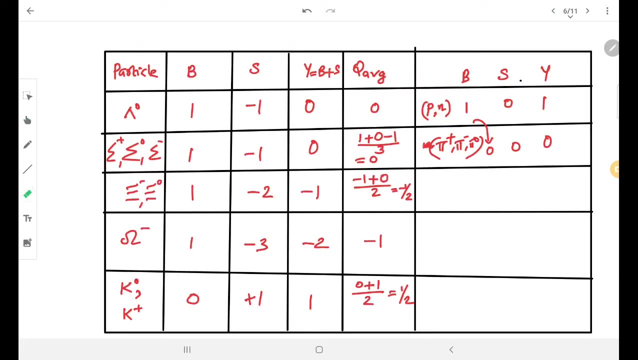 Let us verify this relation. Earlier we said: Let us look at sigma family, Let us look at the example here. For example, Let us look at Psi family. Ok, So We have already Seen the psi family Q average. 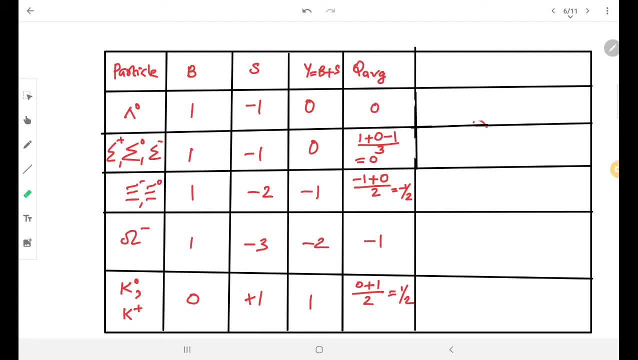 Earlier we said that If we look at the tiroid In the, the 자�, The average allowed. Let us check. Ok, Let us say In this minus 1 by 2 into 2.. So minus 1.. 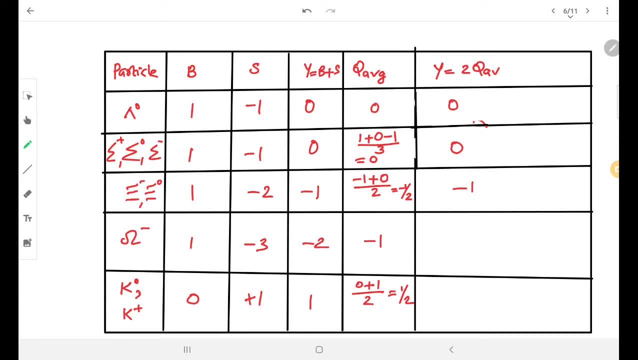 I am multiplying 2 with Q average and forming this table: Here minus 1 into 2, minus 2.. Here 1 by 2 into 2, 1.. So you can see, in this case, that is, we got the same values of B plus S when we did twice Q average. 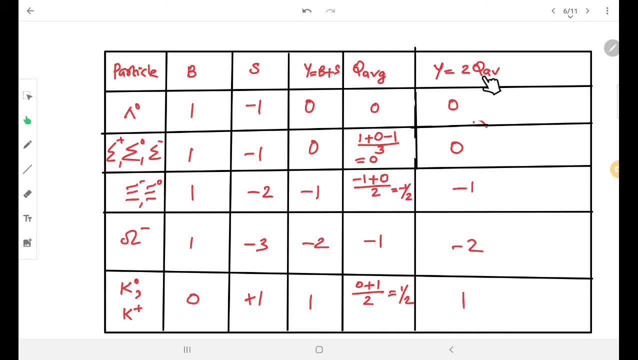 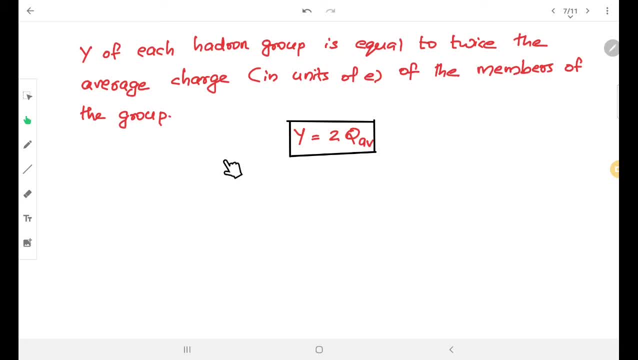 That means hypercharge is actually the average charge of a group twice the average charge of a group. Okay, that is an important relation of hypercharge. Hypercharge is twice the average charge of a particular group. Now we have already seen different examples for this. 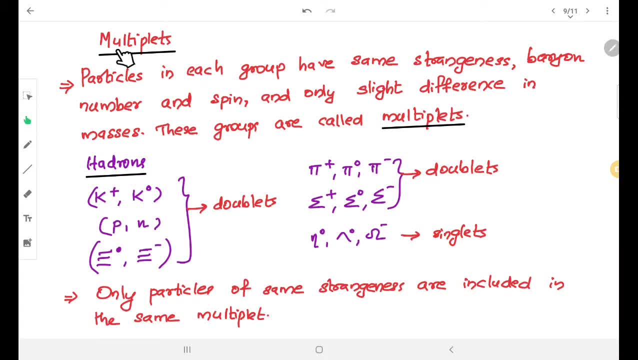 Now these groups are generally called multiplets in particle physics. What is a multiplet? So what is a multiplet Generally? what is the group, What are the properties of that group, Or what are the characteristics of a multiplet? 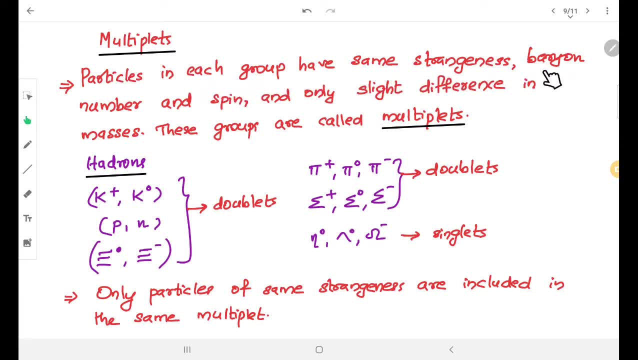 Particles in a group having same strangeness, barrier, number and spin and only same number of particles, So there is a slight difference in their masses. That is what we call as a multiplet. in a group, Multiplets are mainly singlet, doublet and triplet. 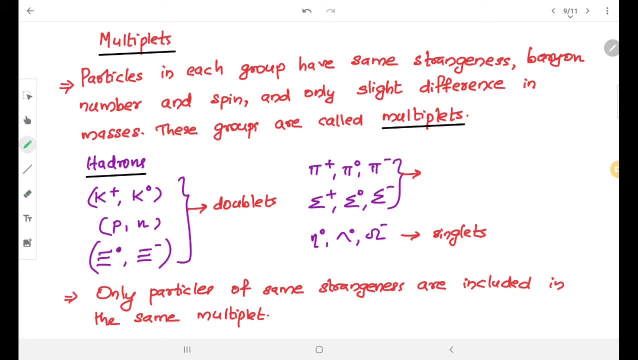 Okay, so these are the categories in multiplets. So let us first see what is a doublet For a doublet. an example is a hand round, a kion. In a kion, there are only two members in the family. So in a family with two members we call them as doublets. In a family with two members they are called baryons and nucleons, Protons and neutrons, Psi-hyperons, Psi-zero and Psi-minus. Now, what do we call a family with three members? 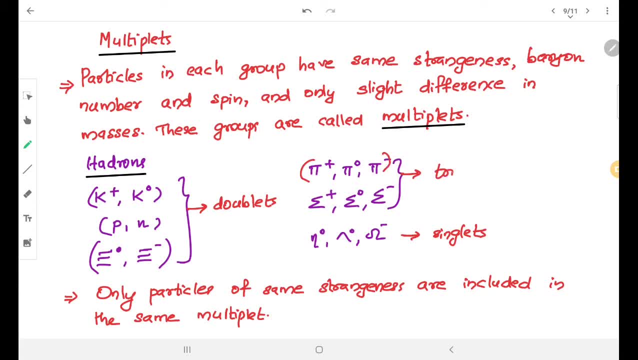 For a family with three members, we call them as triplets. For a family with three members, we call them as triplets Pions. In a family of pions, there are pi-plus, pi-zero and pi-minus. In a family of sigma, there are three members. 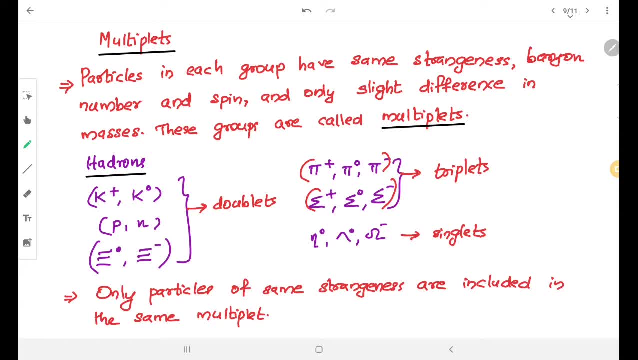 Sigma-plus, sigma-zero and sigma-minus- All of these are triplets. Now next is a singlet In a singlet. there are people who come as singlets, That is, they are themselves In a singlet family. there is only one member in that family. So an example is: eta-zero, eta-mason, lambda-zero, hyperon, omega-minus hyperon. All of these are singlets. So if we take a family, let's take P and N. P and N have a strangeness of zero. The baryon number is one, The spin is half, But there is a small difference in the mass. If the mass of proton is 938, the mass of neutron is 939.. That is what we are told. A singlet is the same strangeness of a group of particles. 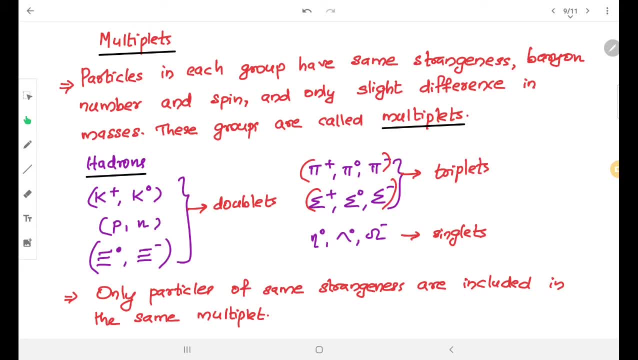 same baryon number and spin, but only a slight difference in their mass. Now, another feature of this multiple is that we can only include the same strangeness- particles- in the same multiple. For example, k-plus and k-zero are particles. Their corresponding antiparticles are k-plus-bar and k-zero-bar, But their strangeness value is minus one. k-plus-bar and k-zero-bar have a strangeness value of minus one, So they do not come in this multiple family. All these corresponding antiparticles form different multiplets. 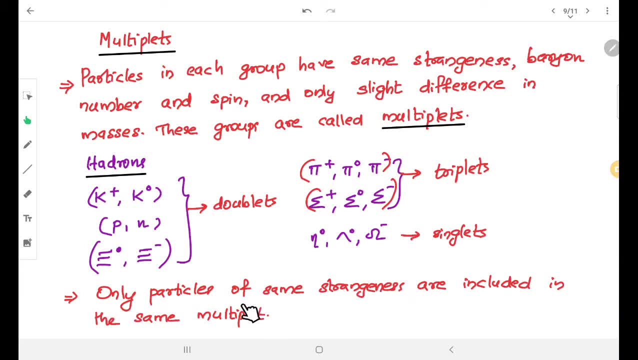 Because they have the same strangeness. So in a group of multiplets there will always be the same strangeness particles, Same baryon number, Same spin particles. So they form in the same group, So they are called multiplets. 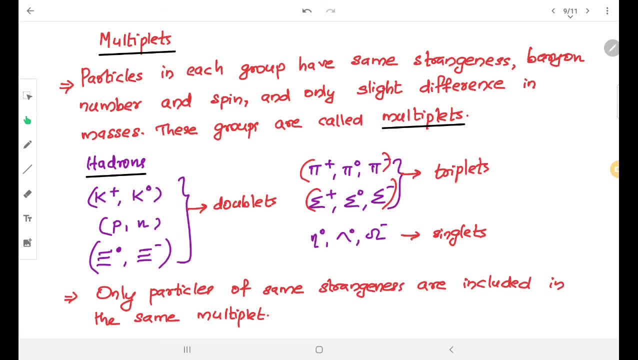 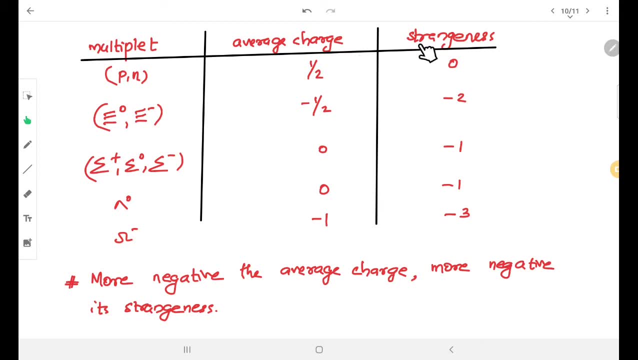 And multiplets can be classified as singlets, doulettes and triplets. Ok, So these multiplets are called the average charge. and strangeness, So this is a nucleon family, This is a doublet, So their average charge is as shown earlier. 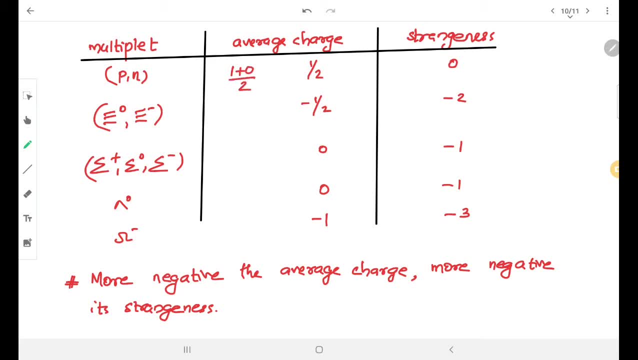 Proton's charge is one, Neutron's charge is zero. So one plus zero by two is the average charge, which is one by two. So this family has strangeness: zero. Likewise psi zero and psi minus. So charge zero minus one by two. 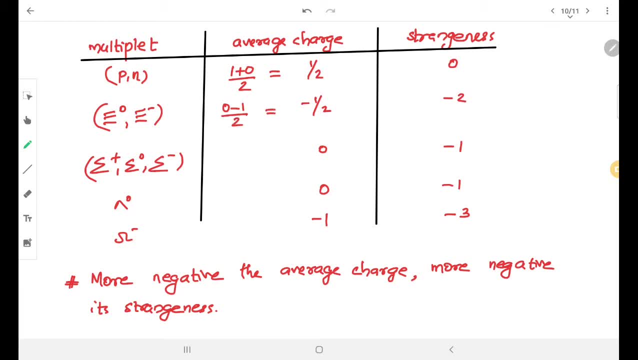 So here minus one by two is the average charge, and strangeness is minus two. Sigma plus sigma zero, sigma minus Charge plus one plus zero, minus one by two, By three, sorry, By three, equal to zero. Then strangeness value minus one. 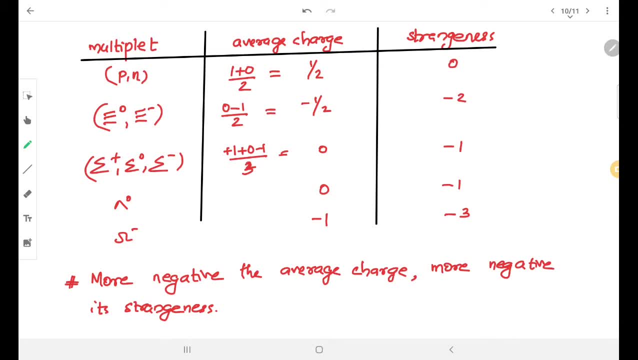 Lambda zero is one particle, Its charge is zero. Strangeness is minus one. Omega minus is one particle. One particle is there, Its charge is minus one. Its strangeness is minus three. So if you look at this form, you can see that 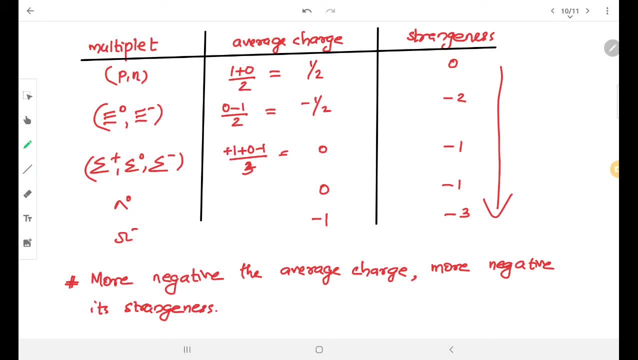 if the value of strangeness is more than or equal to negative, or if the value of average charge is more than or equal to negative, strangeness value will also be more than or equal to negative. So half is a positive value, Then minus 0.5.. 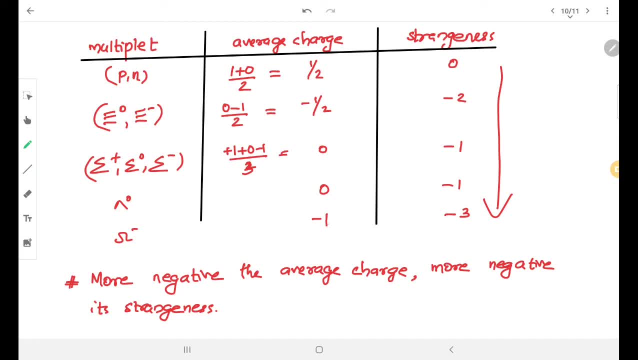 Plus 0.5, minus 0.5, zero, zero minus one. So the highest, largest negative number in this is the negative charge value. The particle is omega minus. According to that, the most negative value of strangeness will be there. 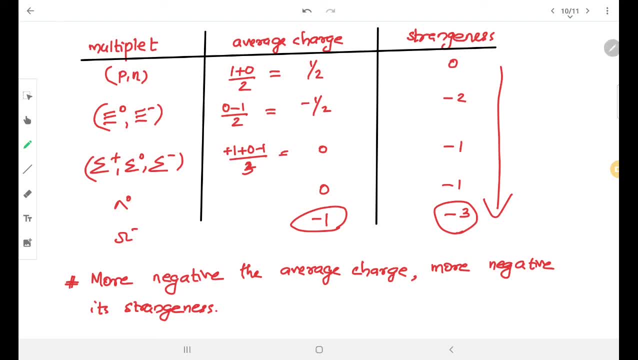 So that is what I have said here: More the negative, more negative the average charge, more negative is strangeness. So this is the relation between hyper charge and the average charge and multiplets. So we have discussed what hyper charge is. 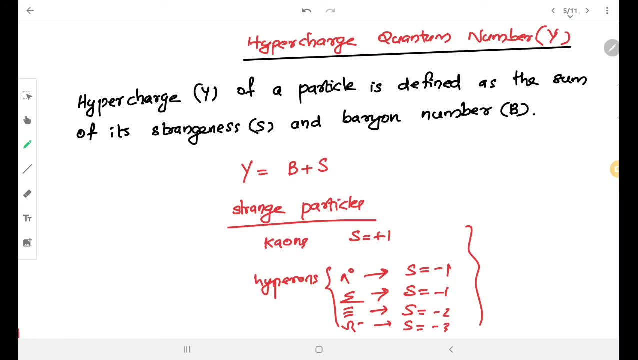 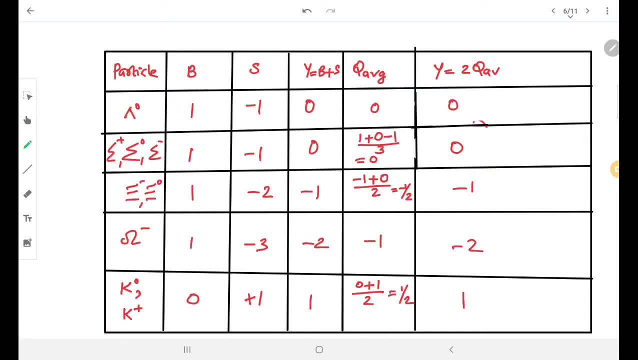 What are its properties? Hyper charge is simply the sum of, it is a quantum number, which is the sum of barrier quantum number and- strangeness- quantum number. So we have seen how to calculate y equal to b plus in each particular case. 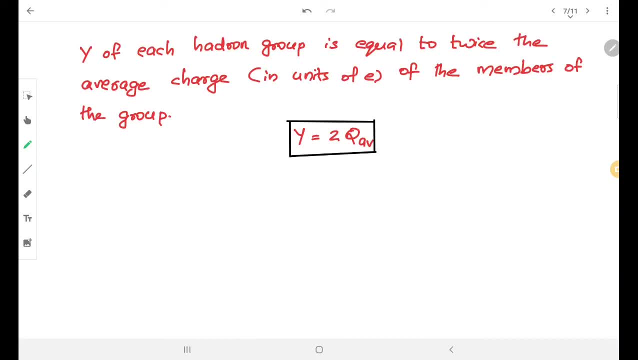 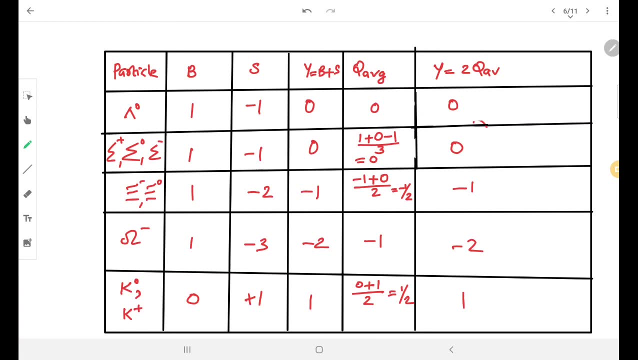 Then the relation between average charge and y is y equal to 2q average, So we can find the average charge in each case. So we have verified that y equal to b plus and y equal to 2q average are equal. 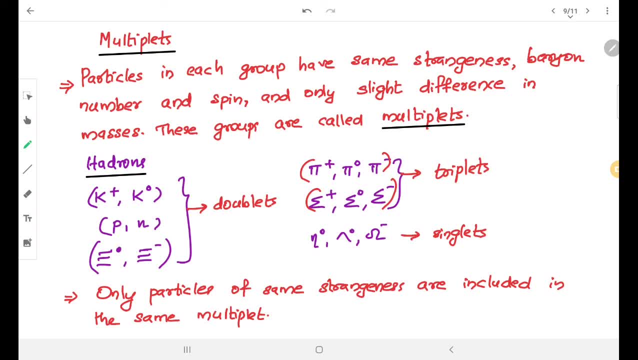 Now we can discuss about. we have already discussed about multiplets. The properties of multiplets are classified as singlet, doublet, triplet. What are the properties of multiplets? They have same strangeness, same barrier number and same spin. 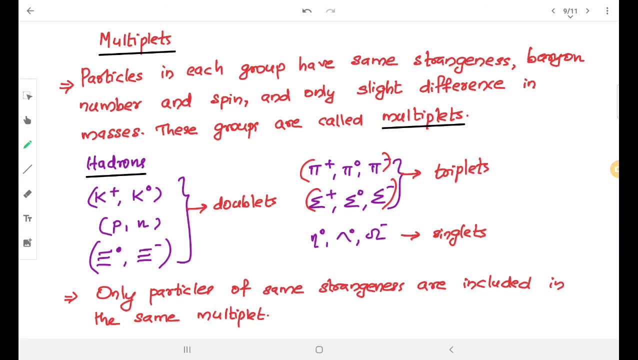 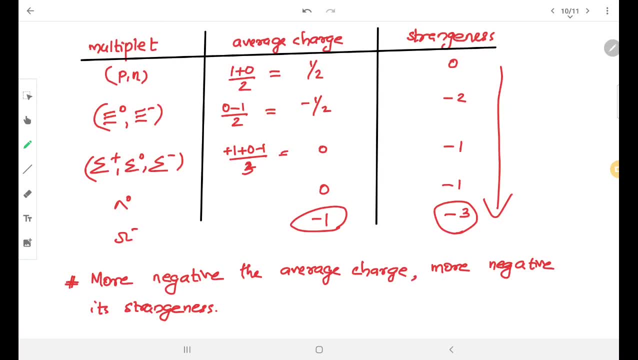 but only difference in slight difference in masses. So in one multiplet family, the same strangeness: members will always be present. So we have seen the corresponding average charge and strangeness of multiplets. Now we have understood that. 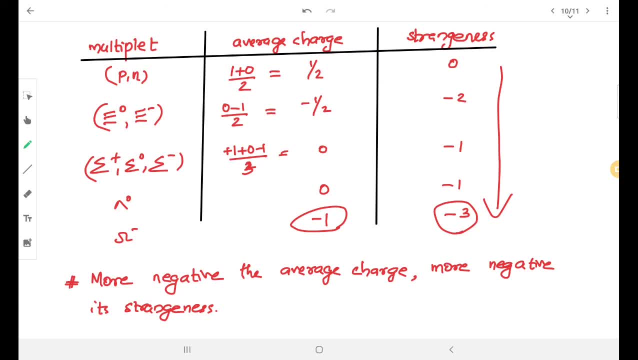 according to: the more the average charge is negative, strangeness will be more negative. Okay, So in the coming class we can discuss about another quantum number. Okay, Thank you.